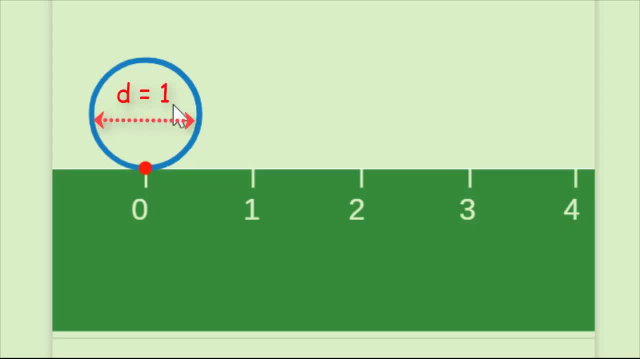 he discovered. Here I have a circle with a diameter of one and it's been painted along the edge or along the circumference with blue paint. Now I'm going to roll my circle along this number line here and see where the blue paint ends, and that will tell me what my 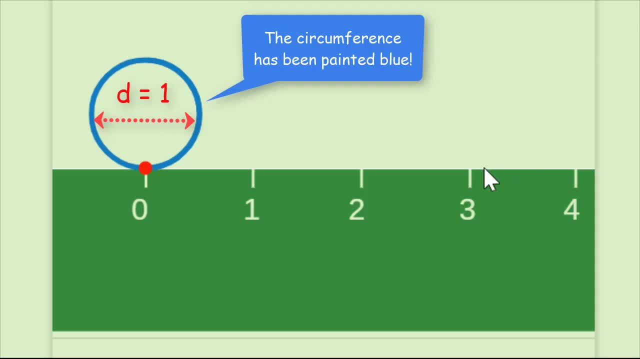 circumference is. and once I know my circumference, I want to know the relationship between the diameter of my circle and the circumference of my circle. All right, so I know my diameter is 1.. I'm going to unroll my circle. That's the length of our diameter. 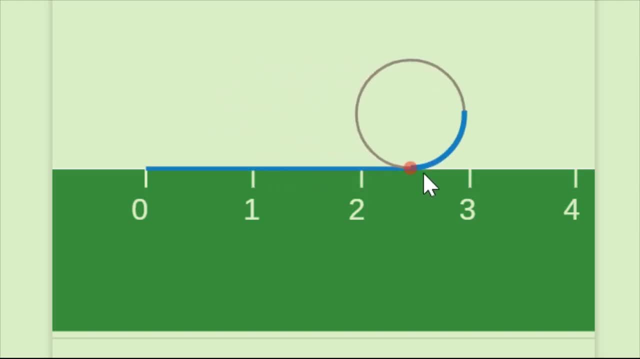 1.. So we're going past that, We're getting all the way to 3. And we have a little bit more. So this distance right here where my blue paint ends, that's the circumference of my circle And it is a distance of 3.14.. So this tells me. 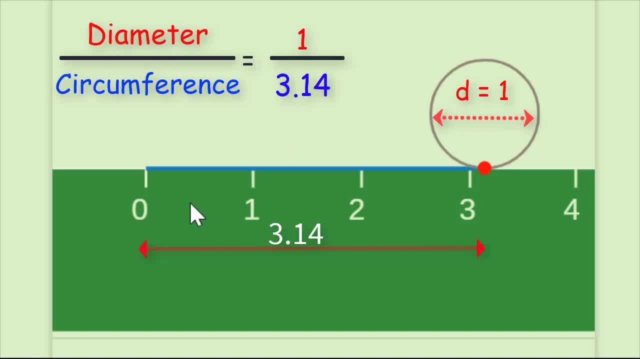 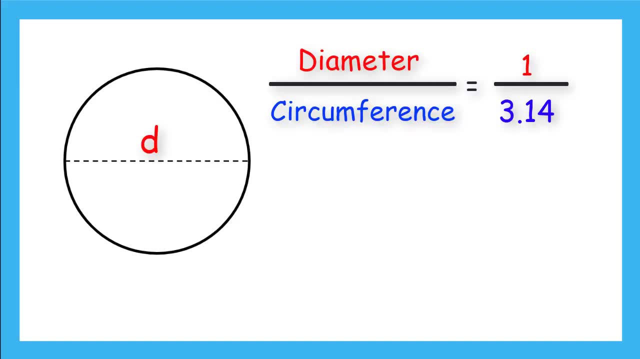 that the relationship between my diameter and my circumference is 1 to 3.14.. Now that we know the relationship or the ratio between diameter and circumference, we can come up with our formula for circumference. We discover that the diameter times approximately 3.14 equals the circumference. But there 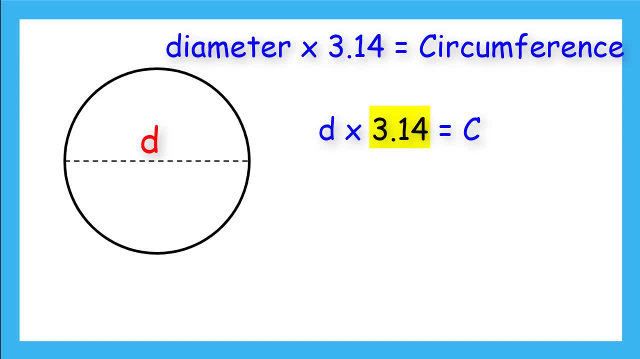 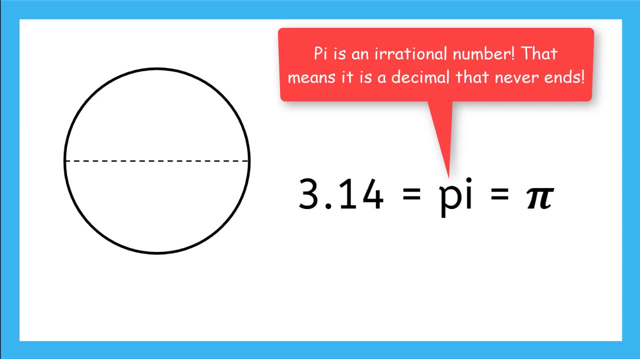 is something special about the number 3.. 3.14.. We call it pi And we use this symbol to represent it. Pi is actually an irrational number. That means it is a never-ending decimal. The numbers just keep going on forever. But we can shorten it to 3.14 and this gives us a very 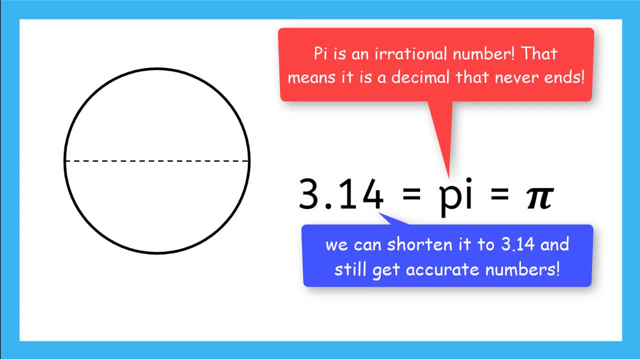 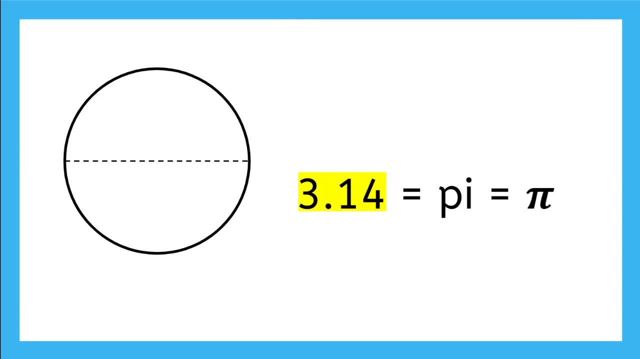 accurate calculation for circumference. Sometimes calculators have a pi button that uses more decimal places in calculations. This is good for very precise measurements, But for us we will just use 3.14. So we can write our formula as C. the circumference is equal. 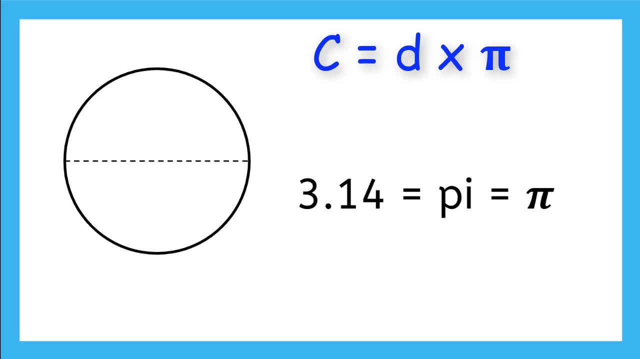 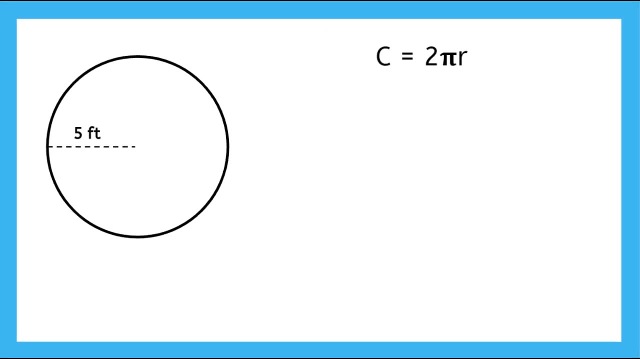 to D, the diameter times pi. I can also plug in the radius, Because we know D is equal to 2r. we can also say C is equal to 2 times pi times r. Now let's do this example of finding the circumference of a. 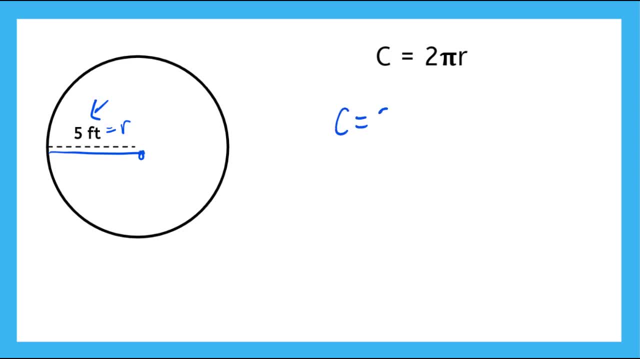 circle. So I have this distance that is given to me, And since it goes from the edge to the center of the circle, I know that this is equal to my radius r, So I can plug it into our formula here. Surcumference is equal to 2 times pau times my radius, which is 5 feet. So now if I multiply my 2 and my 5 together, I get 10 feet, and I am multiplying all of that by pi. And if I look andCO contar all of this and I am multiplying 5 feet with the b Palin and I get IT. I'll show you the way it looks and I'll show you how. 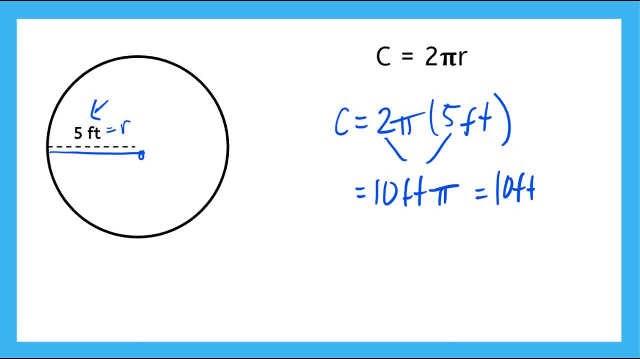 and 10 feet times. remember, pi, we can say, is equal to 3.14. here and now, if I multiply 10 feet by 3.14, I get 31.4 feet, and that's the circumference, or the distance, all the way around my circle. nice work now to find the area of a. 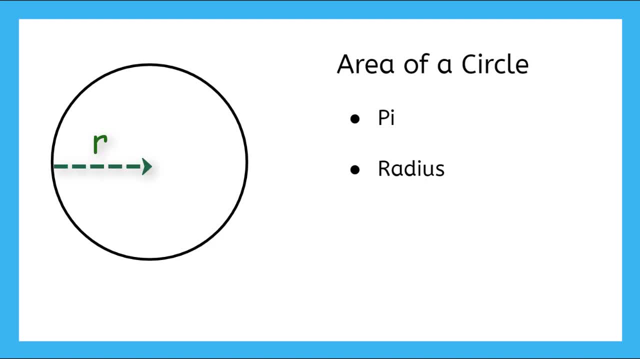 circle. we need to know pi and the radius of the circle and we can use the formula: area equals pi R squared. remember that squaring a number means multiplying that number by itself. so let's do this example for finding the area together. so I have this distance given to me here which goes to the center of my circle. so 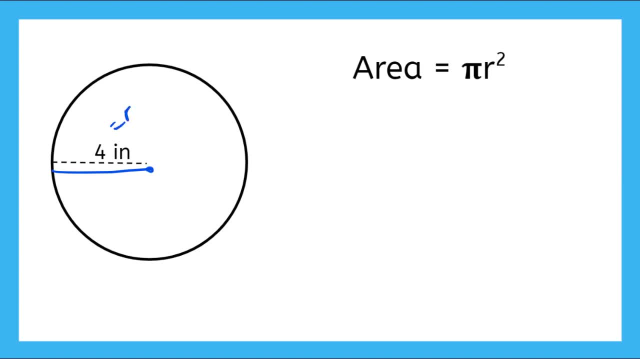 I know that this is equal to my radius R, so I can play that into my formula here. area equals pi, R squared, so I can multiply that by itself. so I can play that into my formula here: his equal to pi, and then my radius, which is 4 inches squared, and so now this is telling me I have 4 inches times 4. 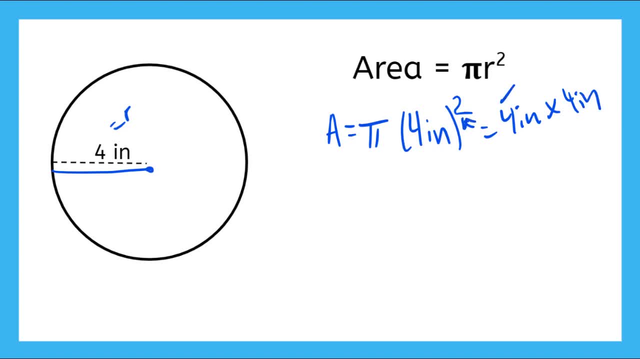 inches. that's what my squared means. so if I multiply my 4 together, I get 16, and if I multiply my inches together, I get inches squared. so now I have: a is equal to pi times 16 inches squared. and if I multiply three point two engaged.